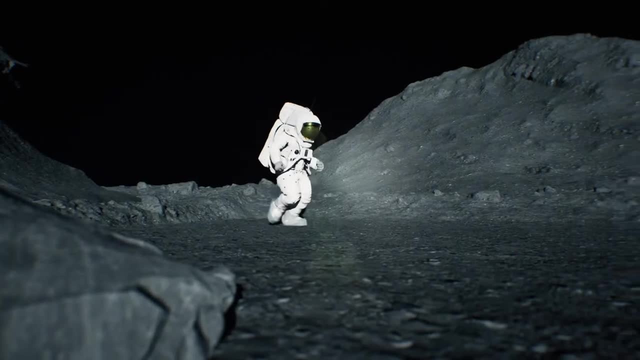 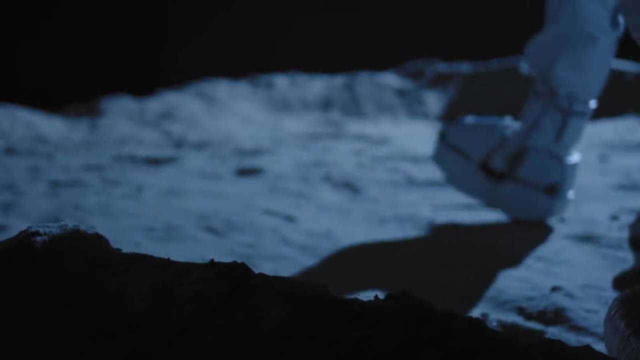 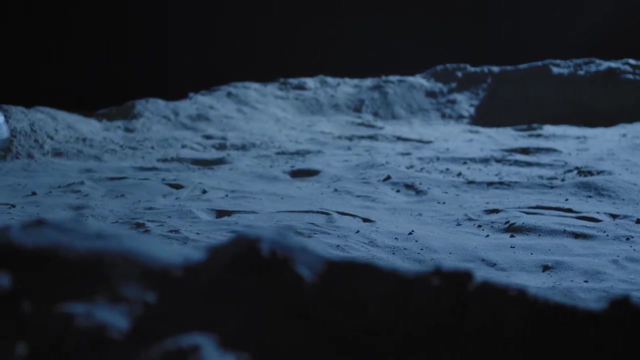 Hello fellow aspiring astronomers, Have you ever heard the quote that's one small step for man, one giant leap for mankind. The famous astronaut Neil Armstrong said this in 1969 when he took his first step on the moon. That quote makes me think about our 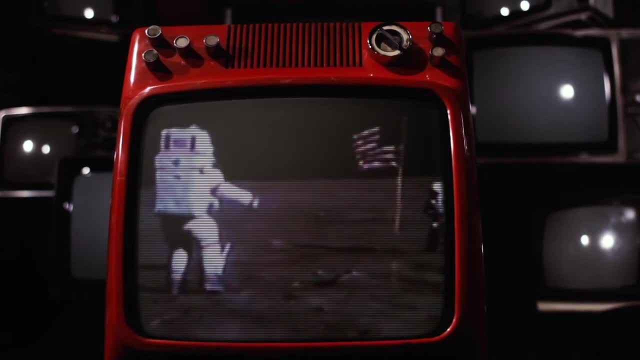 lesson for today. Each step that scientists, mathematicians and philosophers took throughout history to learn more about space led us to where we are today and, thanks to the hard work of astronomers, are leading us to where we will be going in the future. Today we are going. 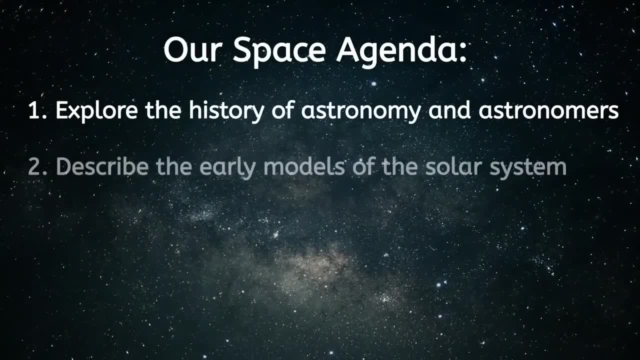 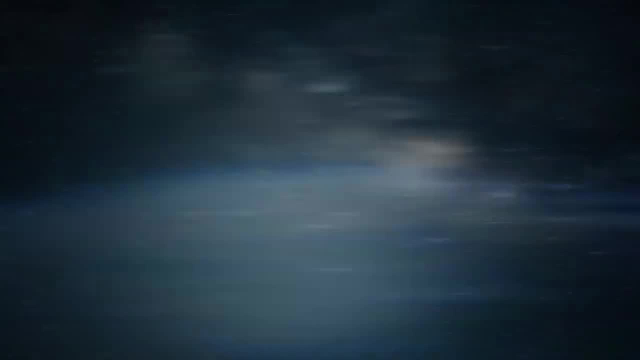 to explore the history of astronomy and those who studied it, describe the early models of our solar system and discuss how we have established our current knowledge of space and Earth's place in the universe. So let's buckle up, because this spaceship is ready to go. 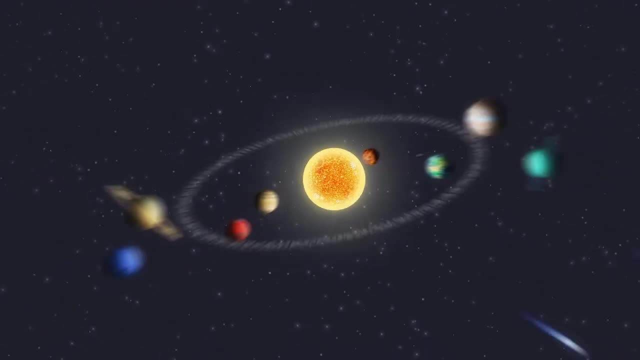 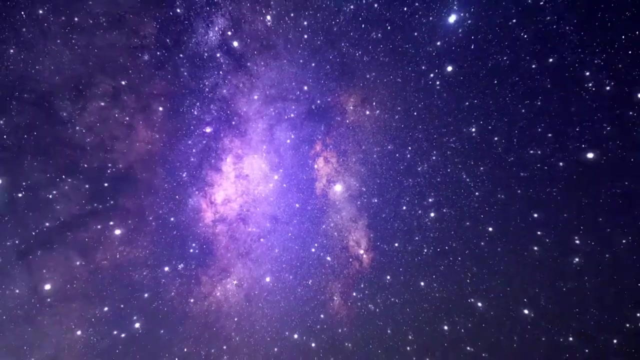 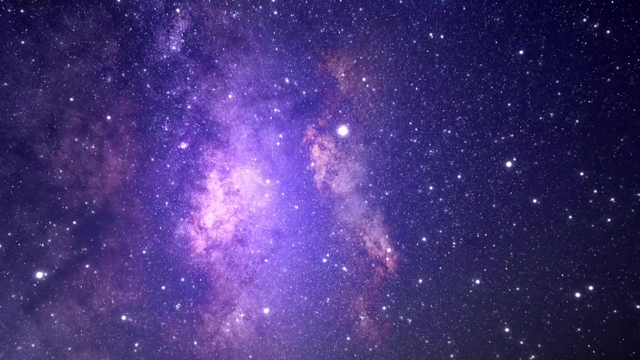 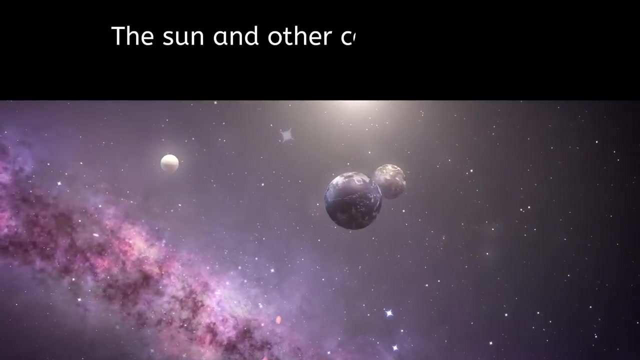 Welcome back, my fellow space explorers. Before we start talking about astronomers, let's take a minute to talk about our solar system. So what is the solar system? Well, it's the sun and other celestial bodies or things in space that are in its orbit and revolve around. 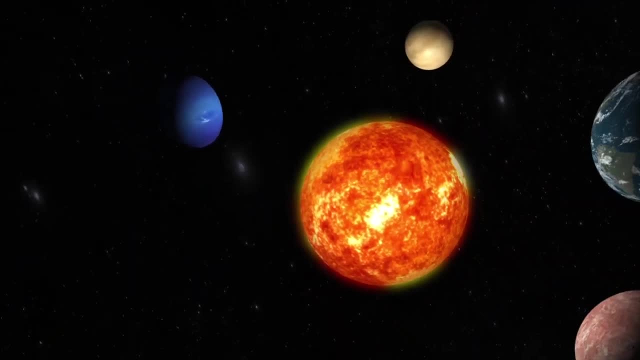 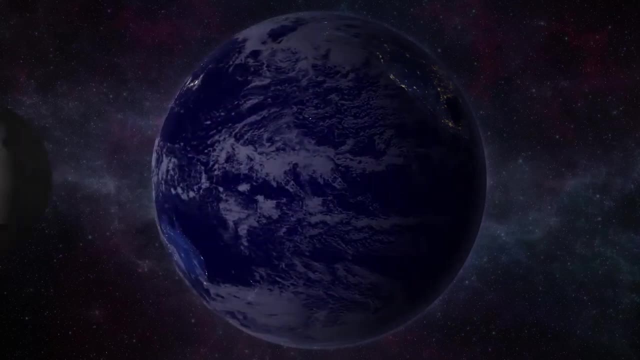 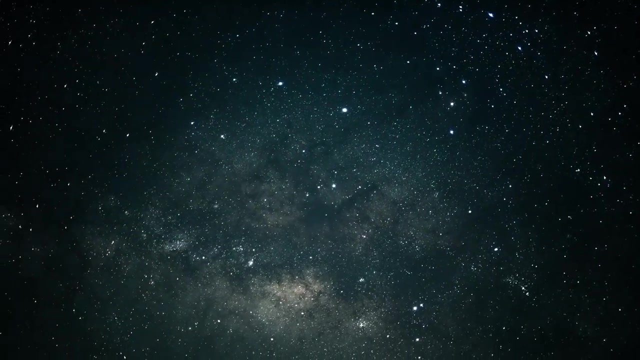 it. Most giants, planets, including the earth, smaller dwarf planets and millions of pieces of rocks and ice orbit our sun. Moons can also be found within the solar system. They are held in orbit around planets by gravity. So how did we come to know all of this? Well, we have to go back to the 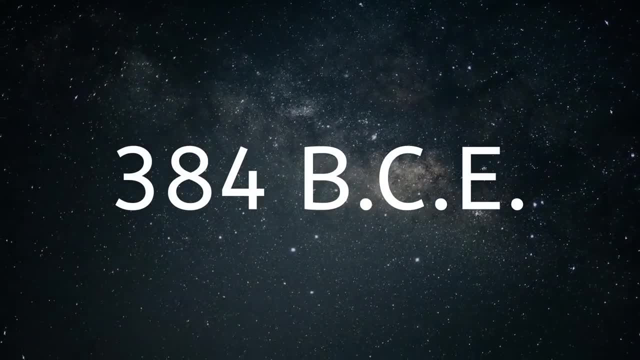 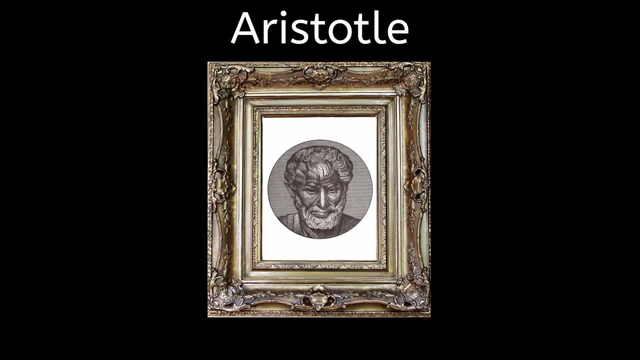 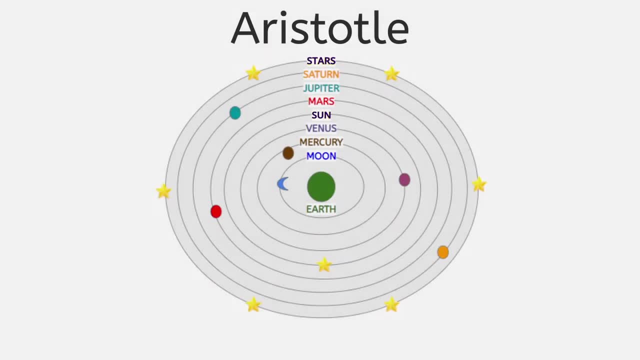 was the center of all things. His model of space placed the Moon, Sun, other planets and stars all orbiting Earth. He thought that if Earth went around the Sun then the relative positions of the stars would change as Earth moved. Aristotle thought that Earth did not move. This may seem. 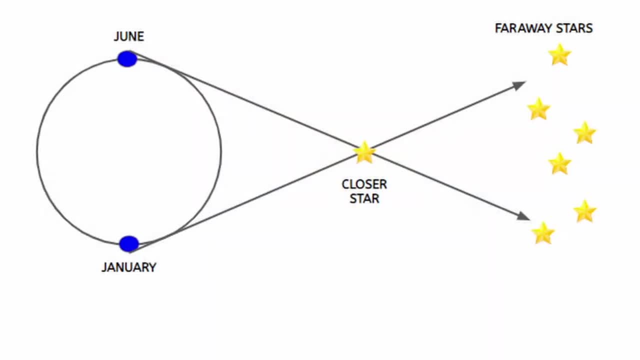 silly now, but there were no telescopes when Aristotle lived. He and other scientists looked for a parallax or a shift in the positions of celestial bodies when they stood at different points on Earth, But they could not see any change. This is because the stars are so far. 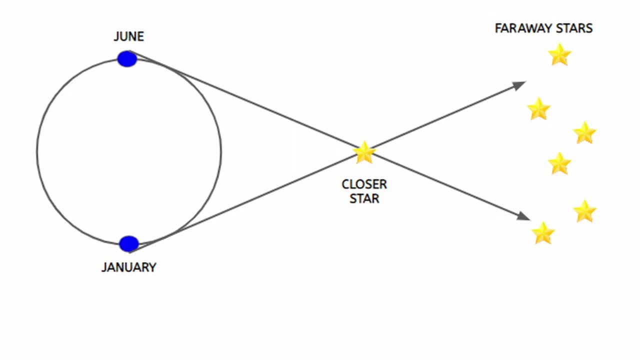 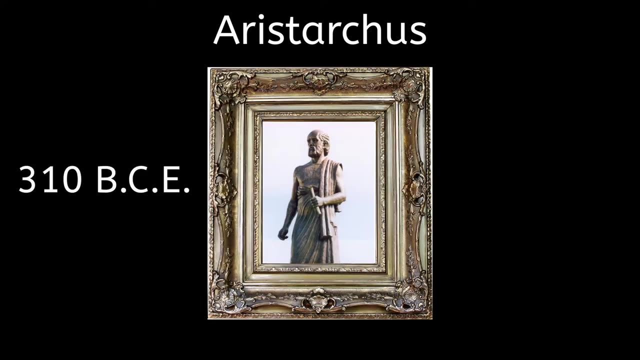 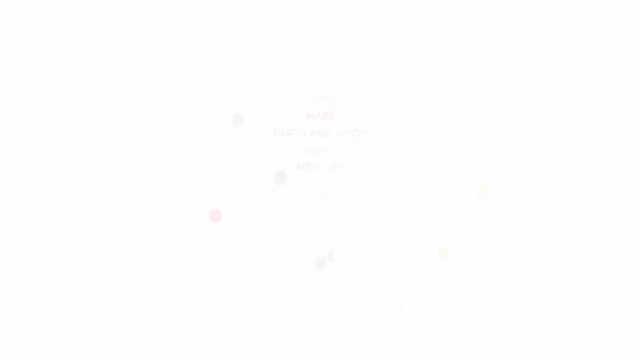 away from Earth, that you can only see parallax with a telescope. Maybe you have already heard of Aristotle, but what about Aristarchus, born 74 years later? He was not a Greek philosopher. He was, however, a Greek astronomer and mathematician. He first proposed a heliocentric. 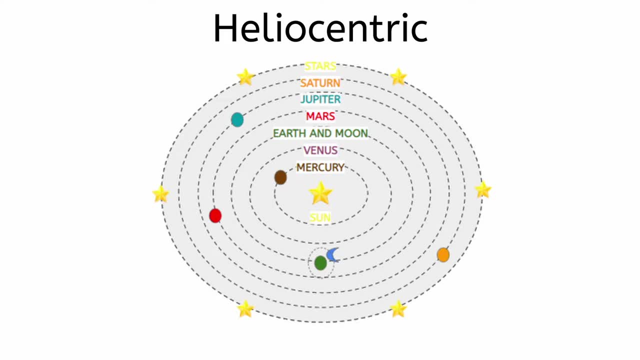 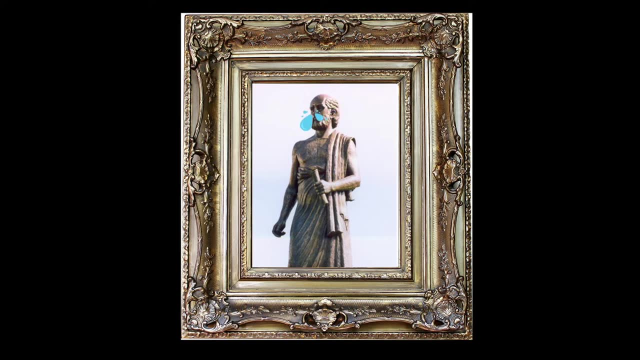 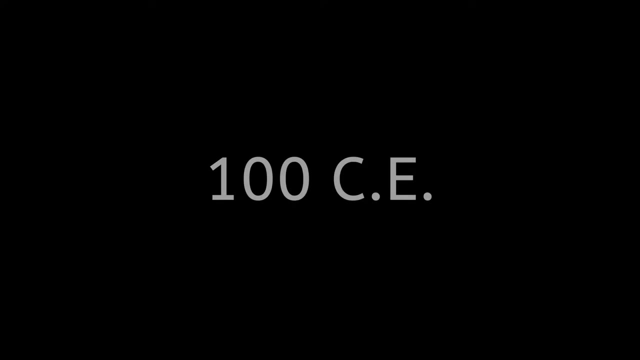 model of the solar system. You know a model of the solar system with the Sun in the center. But, believe it or not, hardly anyone believed him. Come on, people. Now let's jump to the year 100 CE, On Egypt's Mediterranean coast. Ptolemy, a mathematician. 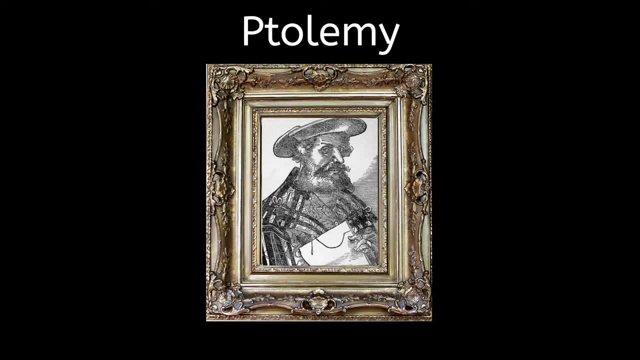 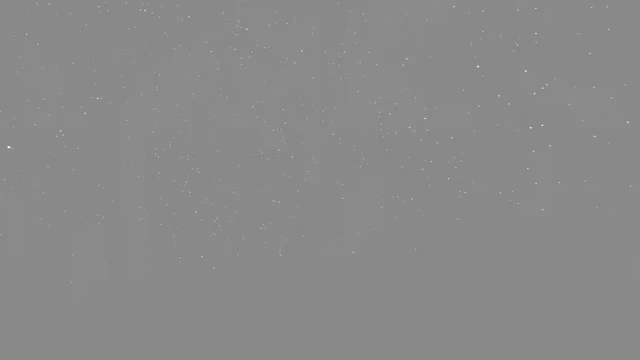 and geographer, studied astronomy and wrote a famous book called Almagest. This book was based on 800 years of observations of the planets. He used these observations to develop a geocentric model, or a model with all the stars. He used these observations to develop. 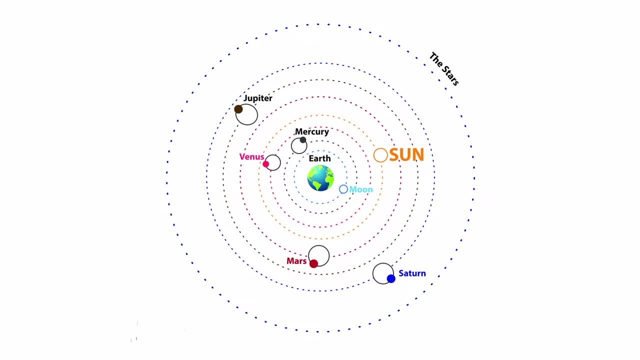 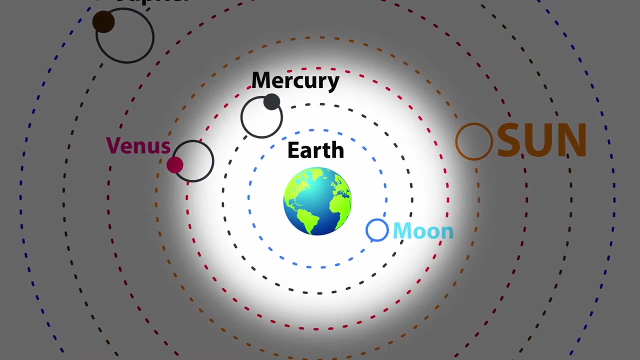 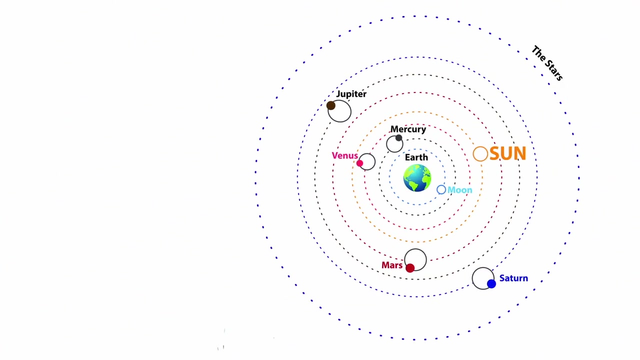 Earth at the center that was used by other astronomers for 14 centuries. Ptolemy believed that planets moved in small circles and they all moved in bigger circles around Earth. and well, it's a lot of circles, Since astronomers followed Ptolemy's model for such a long time. 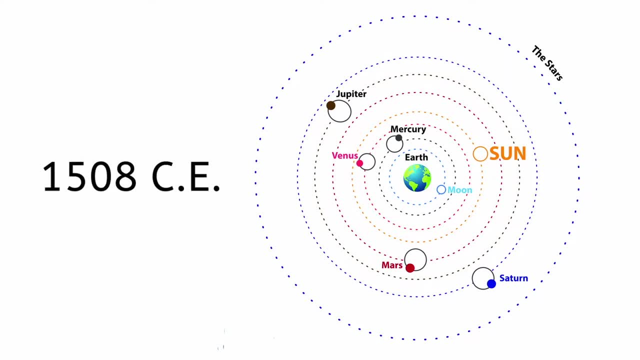 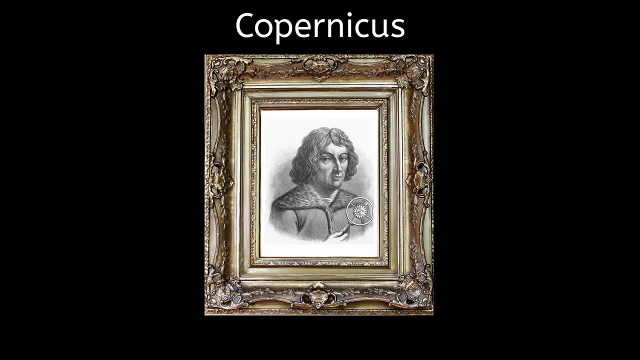 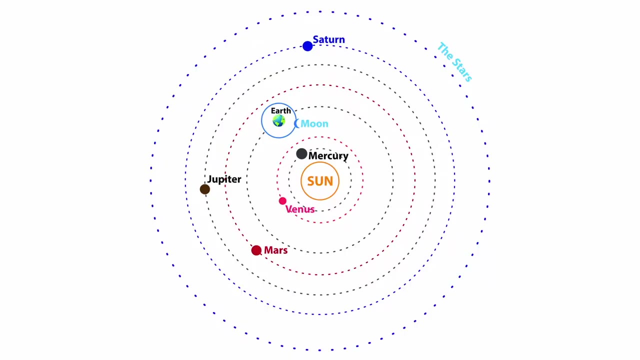 we can jump ahead to the year 1508 CE. This is when Nicolaus Copernicus developed his own model of a heliocentric planetary system, meaning that he believed, like Aristarchus, that the sun was the center of our solar system. However, because astronomers still 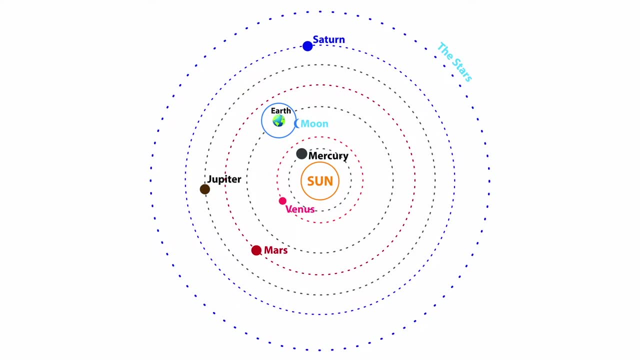 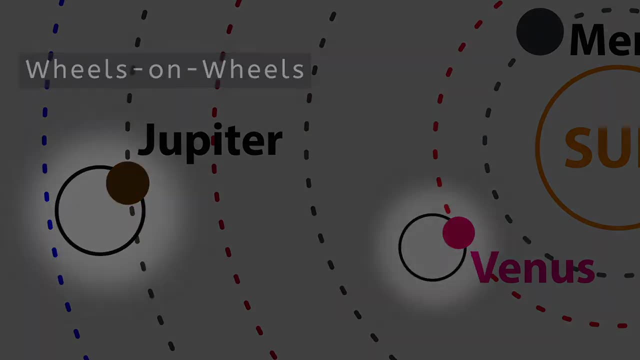 had no special equipment to observe outer space. Copernicus kept Ptolemy's idea that planets moved in perfect circles. This is called the wheels-on-wheels system. Even though he didn't have it all right, the heliocentric model of Copernicus is generally seen as the 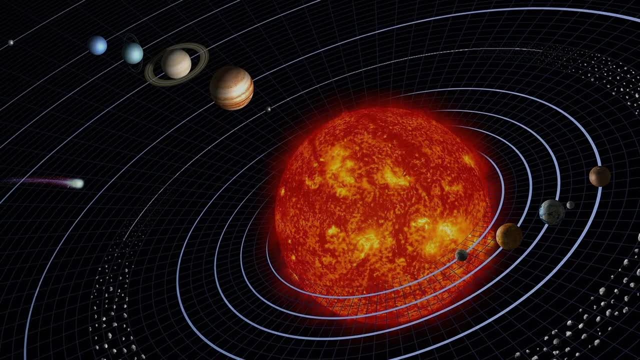 first modern model of the solar system to be developed. A few years later, in 1605 CE, Johannes Kepler, a German mathematician, wrote a book called The Solar System. This was the first modern model of the solar system to be developed. A few years later, in 1605 CE,